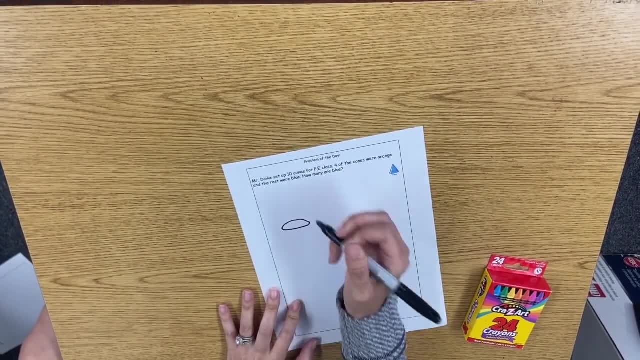 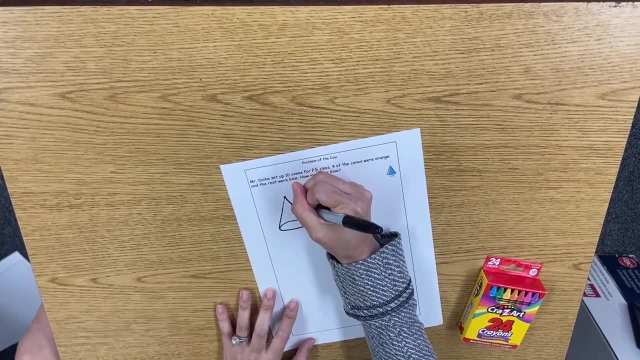 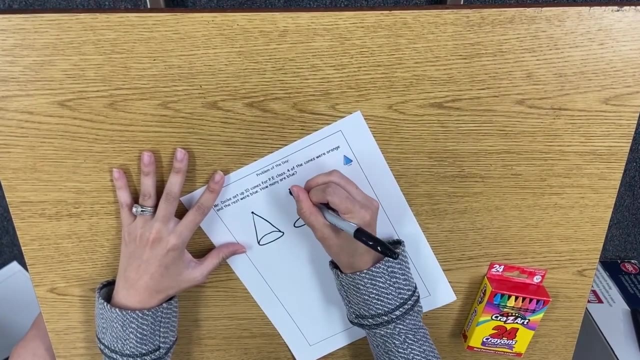 cone you make like an oval, And then I like to make a dot like that And then I connect a line to each side of the oval and that's my best cone. So I need 10 of them, because Mr Doike set 10 of. 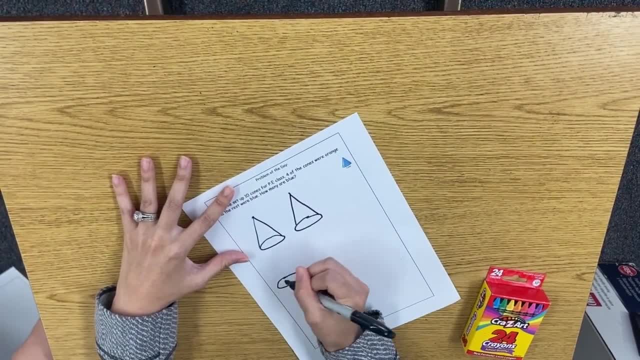 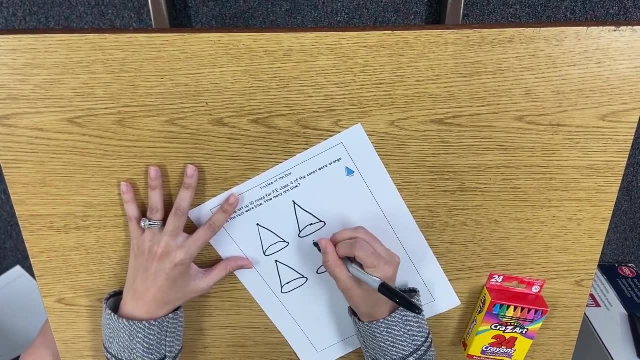 them up for PE. So one, two. so just draw the best you can. So I'm going to draw a line and then I'm going to can take your time, don't forget. if you need to pause my video, you can until you. 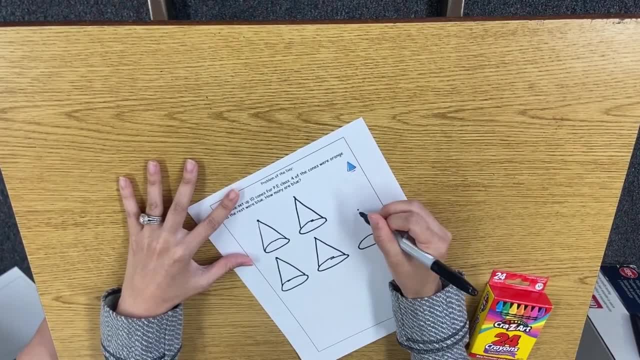 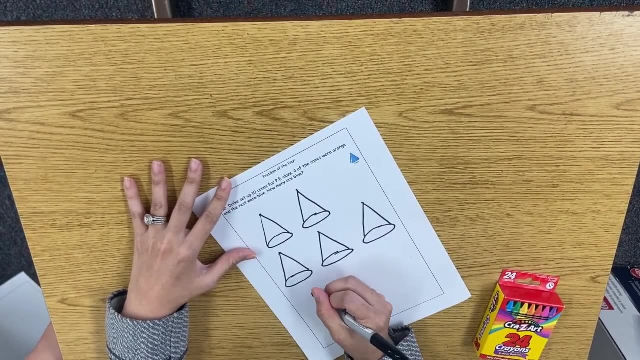 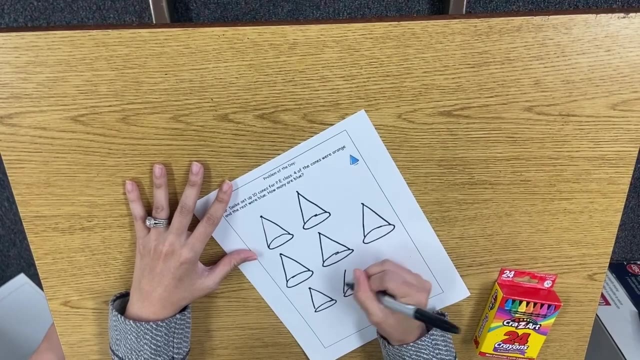 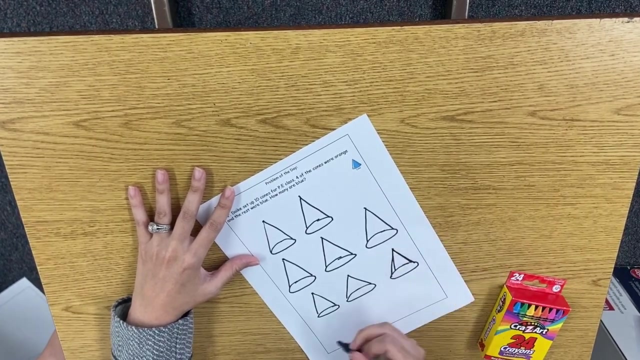 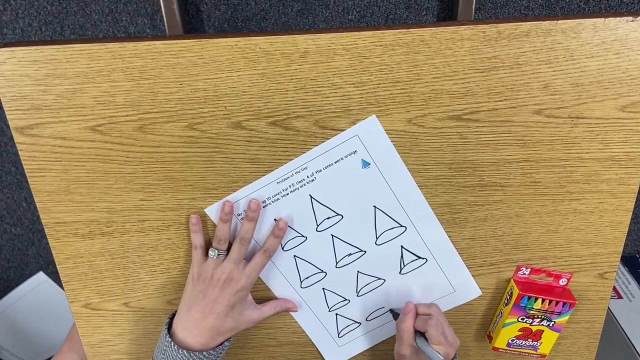 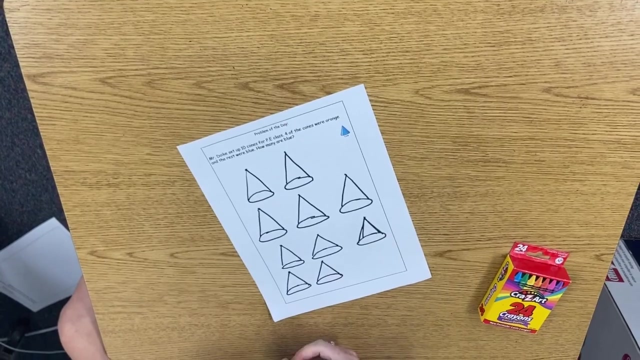 finish drawing your ten cones. so I one, two, three, four, five. I need five more. I'm gonna check my work, make sure I have ten. it's always nice to draw your picture so you can make sure that you have things correct. so I'm gonna check one, two, three, four. 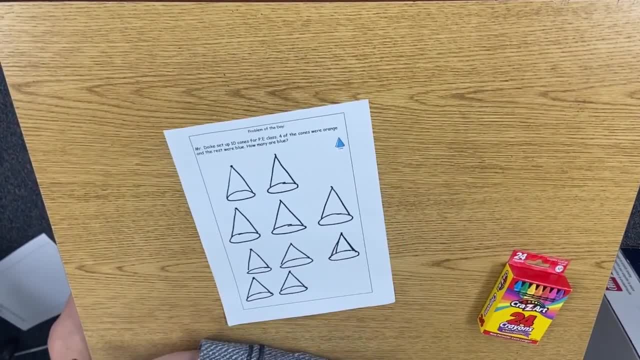 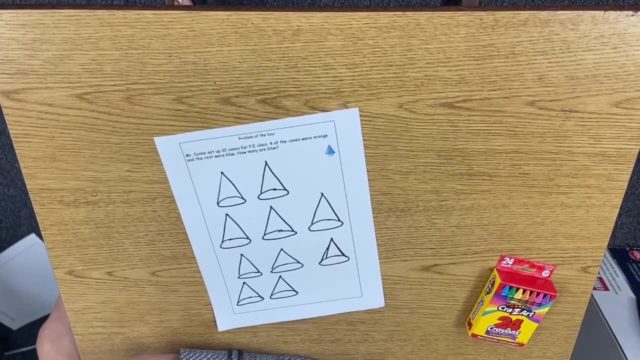 five, six, seven, eight, nine, ten. okay, I draw. I drew the first part of the problem. now let me read the problem again. mr de week set up four cones for PE class. I drew my, I'm sorry. Mr Duique set up 10 cones for PE class. 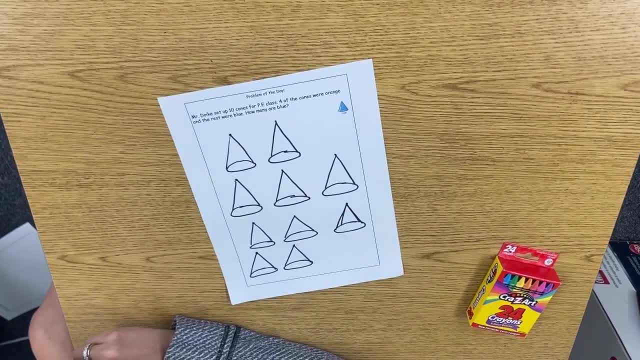 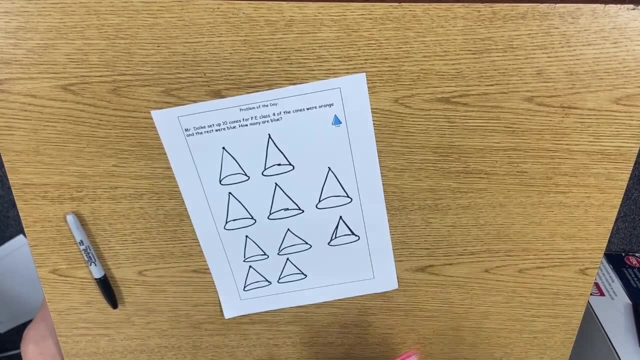 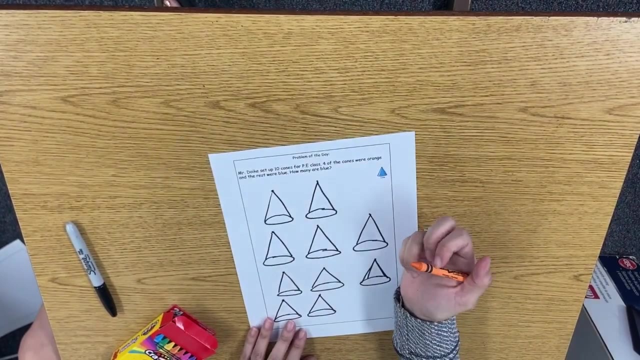 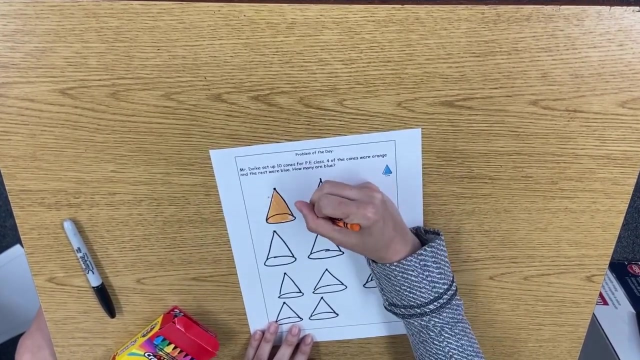 and I just counted my 10 cones. Four of the cones were orange and the rest were blue, And I have to figure out how many are blue. I think what's going to help me figure that out is if I color the four cones orange first. So I want this cone to be orange, this cone, two cones that are orange. 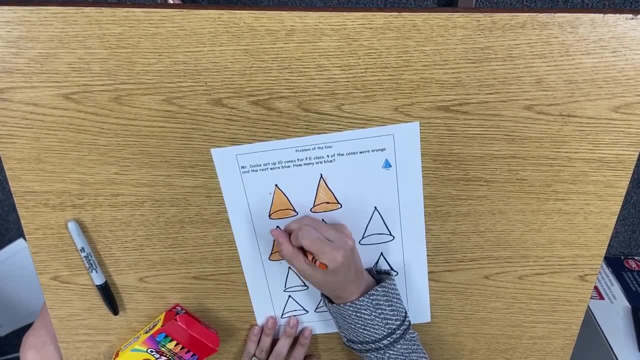 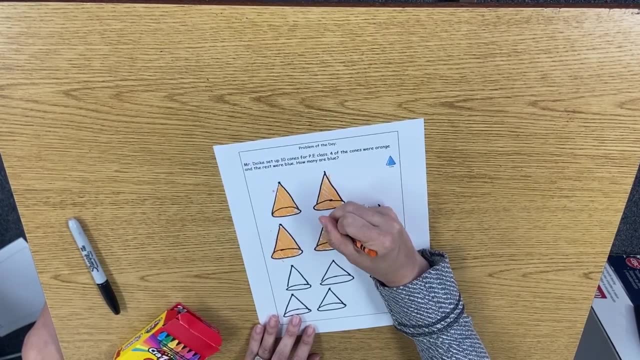 three cones that are orange and four cones. So these four are orange and the problem says: the rest are blue. So I am going to color my 16 cones for PE class. So I'm going to do my orange and four cones right. So I'm going to color my 16 cones for PE class. So I'm going to go ahead and